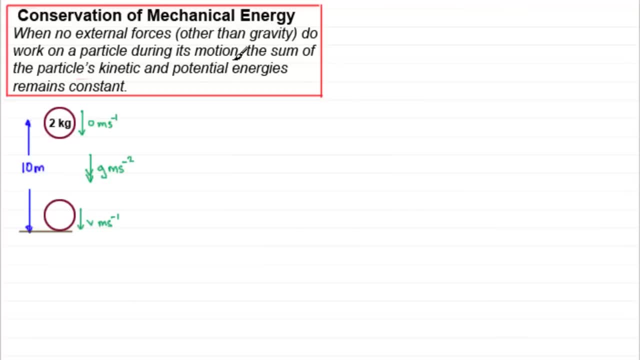 during its motion. the sum of the particles, kinetic and potential energies remains constant. And I can use this principle here, Because if I assume that there's no air resistance, no work will be done against any resistance. We'd just have the force due to gravity acting on our particle. Then I can take two points in this. 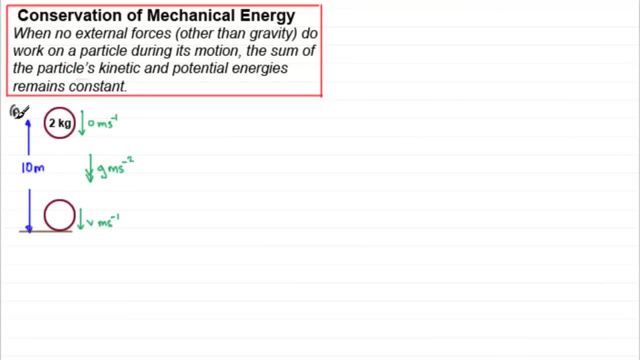 motion. Let's say this point up here, which we'll call A, and this level down here on the ground, which we'll call B. So what the principle of the conservation of mechanical energy is is that you have to of conservation, mechanical energy is saying is that the gravitational 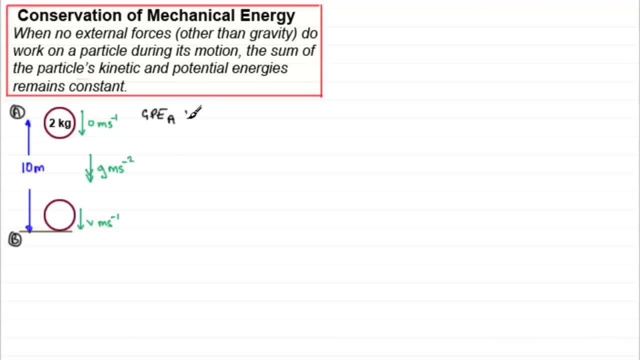 potential energy at A plus the kinetic energy at A must be a constant value, and so, therefore, if it's a constant value, that sum must be exactly the same as you get at B, so in other words, the gravitational potential energy at B plus the kinetic energy at B, and what we can do then is say: well, okay, what kind of. 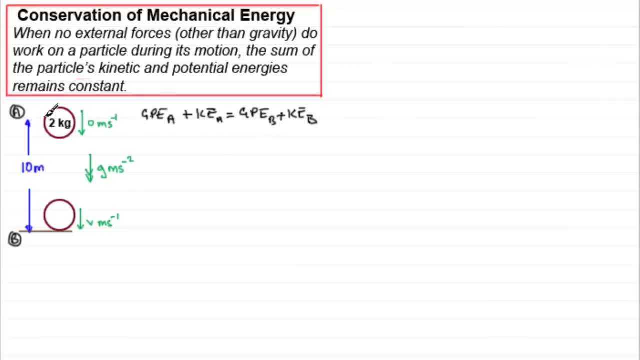 gravitational potential energy does the particle possess at A? well, if we take this as our zero level, then it's going to be mgh, so the mass is 2. so we're, therefore, we're going to have 2 times the acceleration due to gravity, G times the height, h, ten meters. 2 G times 10. now, what kinetic energy does it? 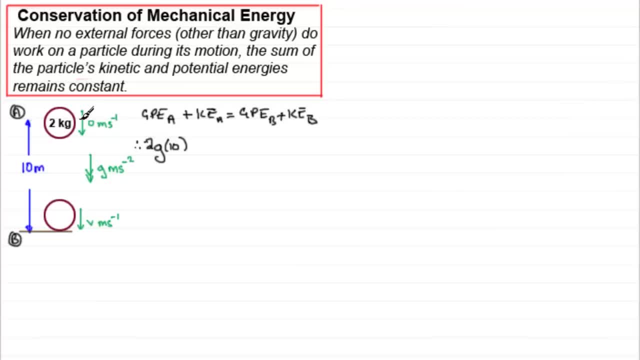 possess up here? well, none, because it's not moving, it's at rest. so this must be equal to the gravitational potential energy at B. but there is none because we've taken this as the zero level, so there's no heights here involved. and then we've got then. the kinetic energy as a function of the potential energy is 0.3 per the moment. 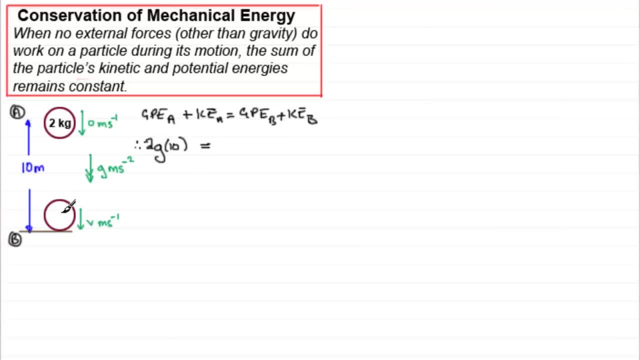 energy at b. So that's going to be a half mv squared. So half multiplied by the mass of two times v squared, Half mv squared. But if we take g to be nine point eight, then what we end up with here is v squared. Let's just put this down on the left, this time V squared. 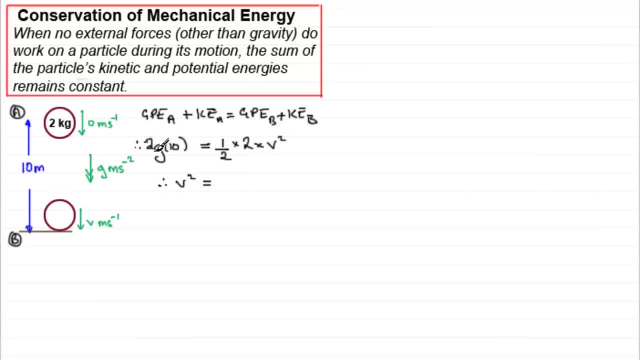 equals, and if you do two g times ten, g being nine point eight, you get a hundred and ninety-six. We can get v by square rooting this. So v equals square root of hundred and ninety-six, and that turns out to be fourteen, Fourteen meters per second. Okay, Now, I did say that. 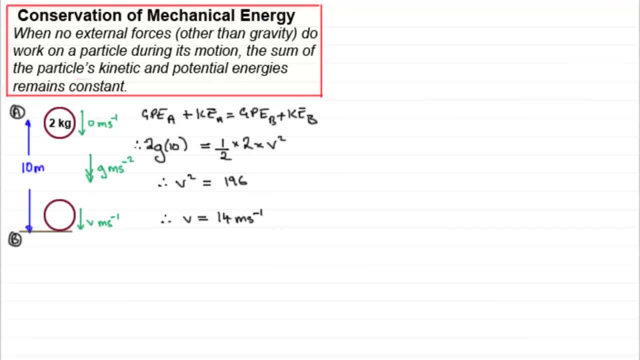 you could have done this just by using our Suvat equation, So I'll run through that and then I'm going to show you how you can do that. Subtitles by the Amaraorg community. Subtitles by the Amaraorg community. S is displacement, so we need to set up a positive direction. 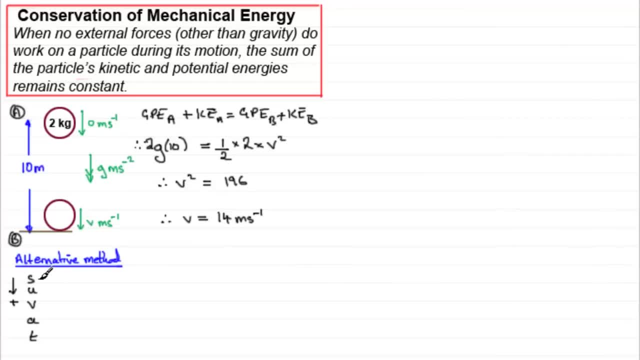 Let's have downwards as being positive. So the displacement would be 10, 10 meters U. the initial velocity would be 0,, 0 meters per second. The final velocity- well, that's what we're trying to find- Acceleration due to gravity is g or 9.8 meters per second. per second. 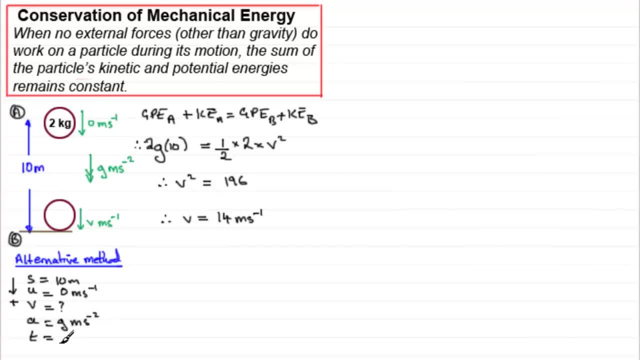 And t. we don't know how long it took to drop from here to here. So, ok, we don't know that result, we'll just mark it with a cross there. So how are we going to find this out? v. Well, clearly, we want an equation that leaves out t. 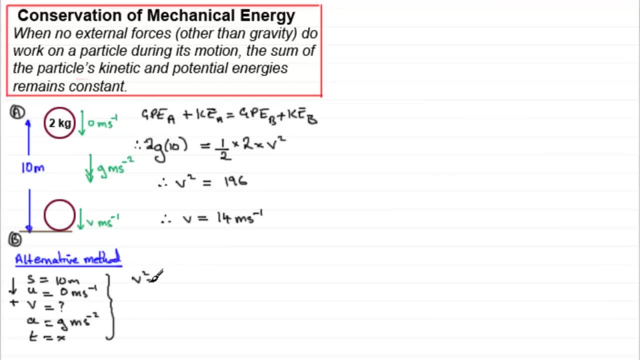 And that's going to be: v squared equals u squared plus 2as, So that's going to mean that u squared is 0, 0, 0, 0 squared is 0, plus 2 times acceleration, which is g Multiplied by the displacement s of 10. 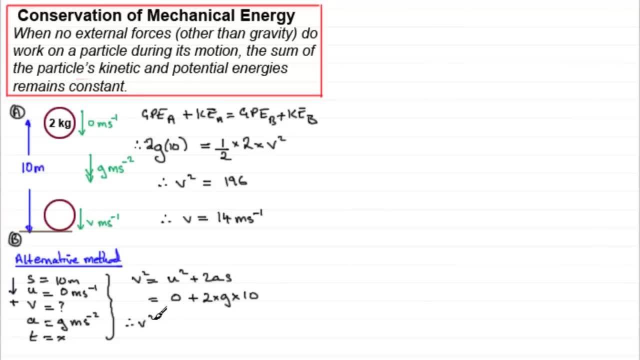 So you get v squared equals 2g times the 10, Comes out 196, take g to be 9.8, And so obviously we get v by square, which is 196, And that comes out at 14 meters per second. Not much in it, really, when you compare these two methods. 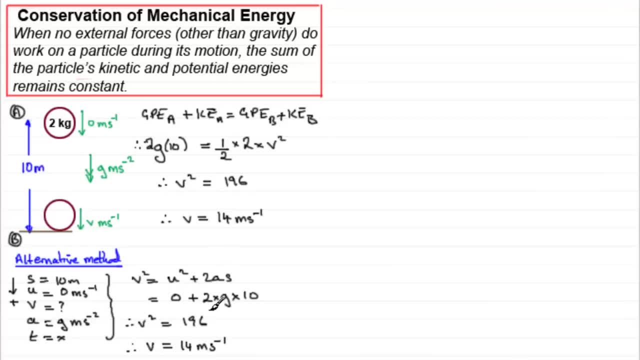 But you'll find later that when we do problems where there's resistance to motion And problems where motion's not necessarily in a vertical line And acceleration isn't constant, We're going to have to abandon this approach. Ok, so that's ok for now, But, as I say, I want to try and introduce you to some other methods. 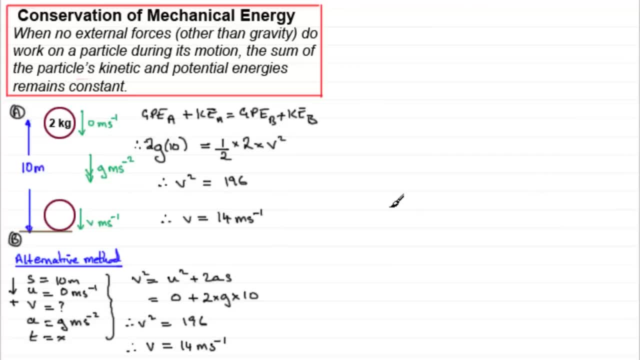 And I want to introduce you to this idea here. Now we could do this problem another way. anyway, It's by something called the Work Energy Principle. It's this principle here That the change in the total energy of a particle Is equal to the work done on the particle. 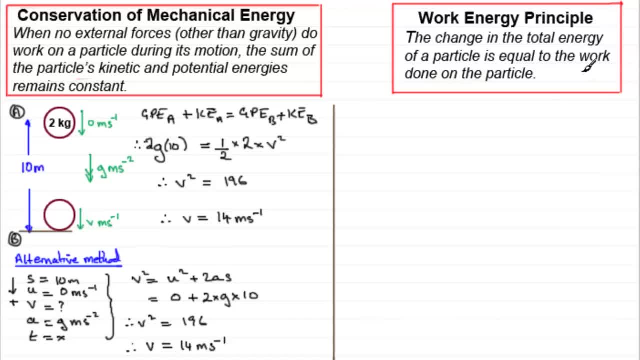 Now, if I use this principle for this question here, What we do is we look at the Gain in kinetic energy first of all. Ok, so we'll just put this down here: Have gain in Ke Now the gain in kinetic energy Is going to be equal to: 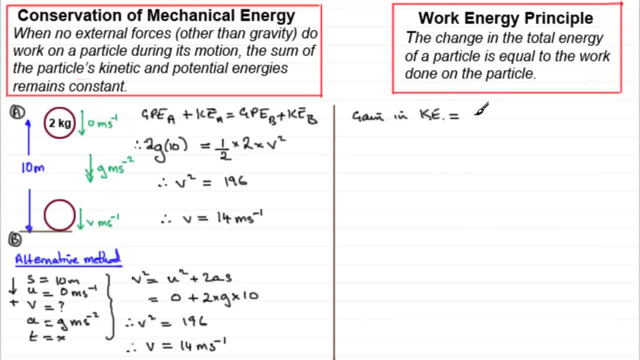 The final kinetic energy minus the initial kinetic energy. Well, we know kinetic energy is a half mv squared, So it's going to be half the mass two Times the final velocity squared. Half the mass two times the final velocity squared. Half the mass, two times the final velocity squared. 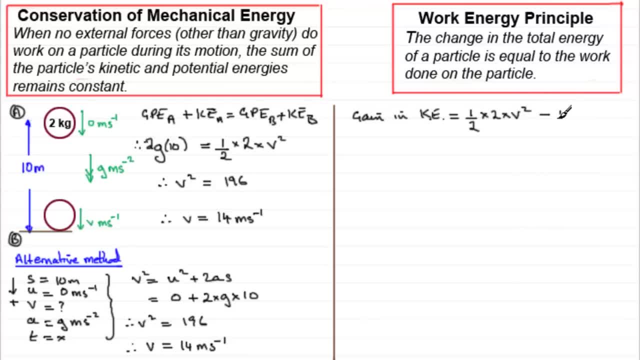 Half mv squared, Minus the initial kinetic energy, Half times the mass times, v squared. But v was zero. So that's going to be zero squared And if you work that out Then it just comes out to be v squared. This term zero. half of two is one. 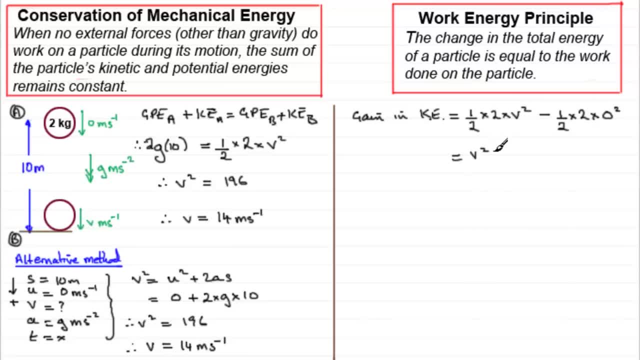 So you just get v squared. Ok, we've got that. That's the gain in Ke: kinetic energy. Now what happens is the particle Drops. it now loses potential energy, Gravitational potential energy. So we talk then of the loss in Gravitational potential energy, GPE. 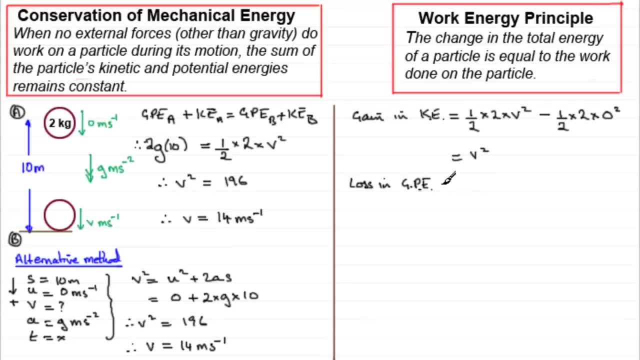 Alright, and so what's that going to equal? Well, we know that gravitational potential energy is mgh, So we've got m being two Times g, nine point eight times h being 10.. What does this come to? Well, it comes to 196.. We should really put. 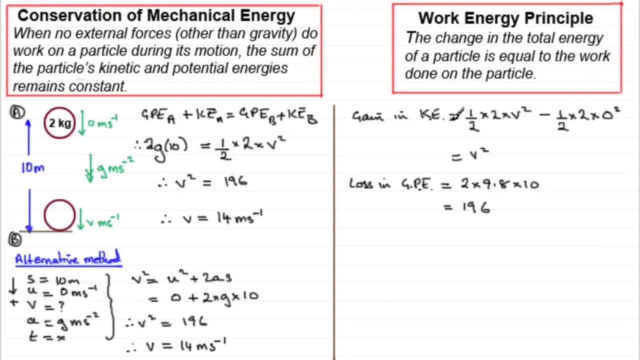 these units in. by the way, I seem to have missed those out: Kinetic energy measured in joules, and the same with gravitational potential energy joules. So now, using the work energy principle we've got. the change in total energy of a particle is equal to. 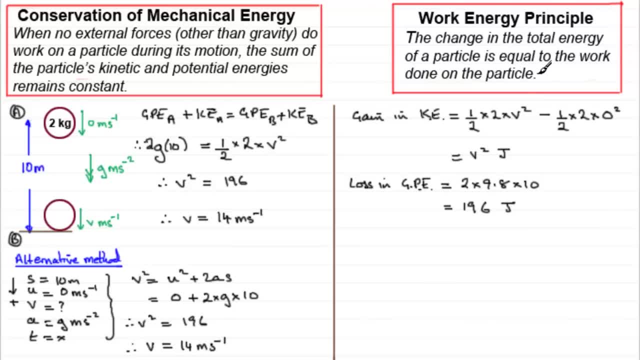 the work done on the particle. So let's have a look. What was that work done on the particle? Well, let's just first of all just write down the change in total energy. we'll just write: just energy here is equal to the work done on the particle. Well, that would. 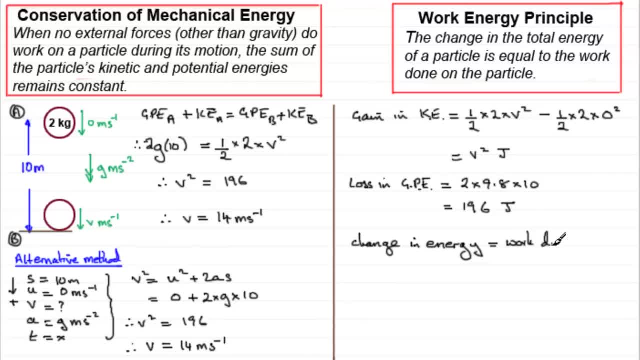 normally be the work done against resistance. Let's just write it in anyway: Work done against resistance. Just drop to a new line there. So what is the change in energy? Well, that's going to be the gain in kinetic energy minus the loss in gravitational. 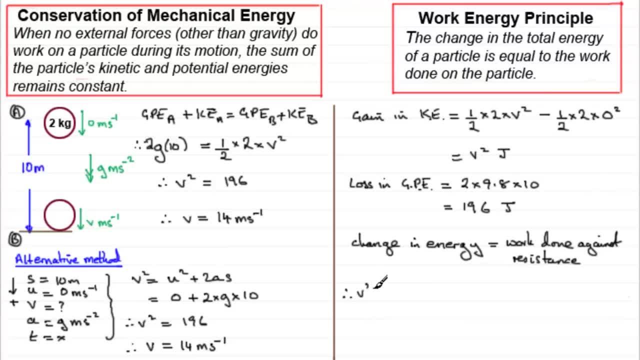 potential energy. So therefore we've got v squared minus 196.. And we're told that that's equal to the work done against resistance. But in a problem like this, if we are assuming there wasn't any air resistance, then this is going to be zero. So it's just 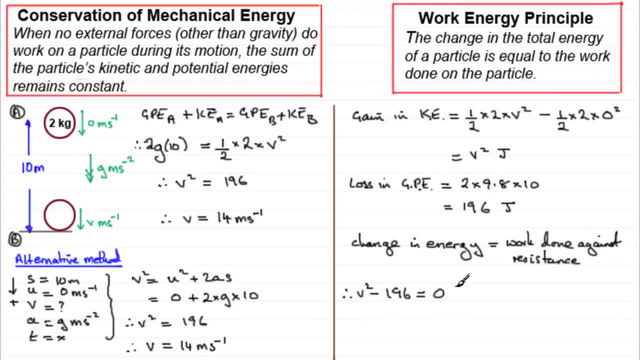 going to equal zero in this one. Later problems, though: when we're doing motion on a rough inclined slope, for instance, there will be resistance friction, So we're going to have to do some examples on this where this won't be zero, But for now it's zero, And so if 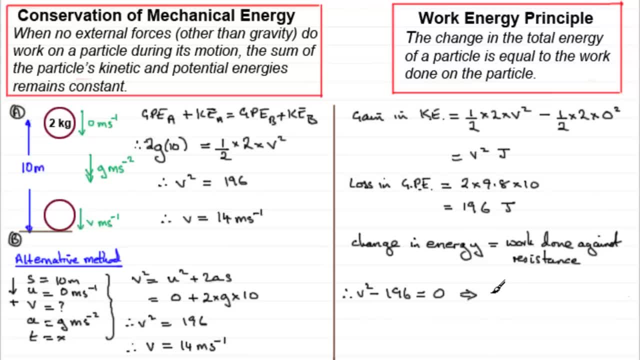 we have 196 to both sides, it follows that v, squared, equals 196.. And then just take the square root and it follows that v equals 14. then meters per second: Same answer as we had before. Now, some people will not necessarily write it out like this either What they'll say. 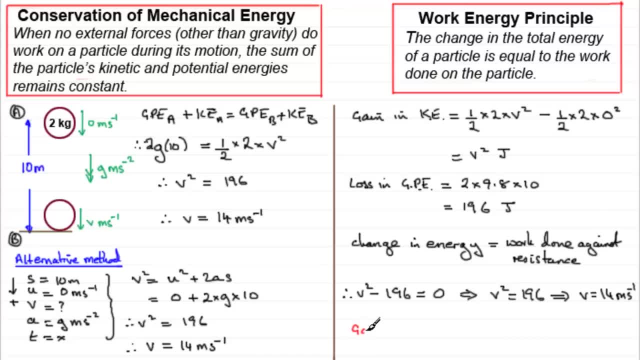 is that the gain? let's just write it down here: the gain in kinetic energy is equal to the loss in potential energy, because there was no work done on the particle. So you might see that given, And that's what we've done here. basically, If you were to write: 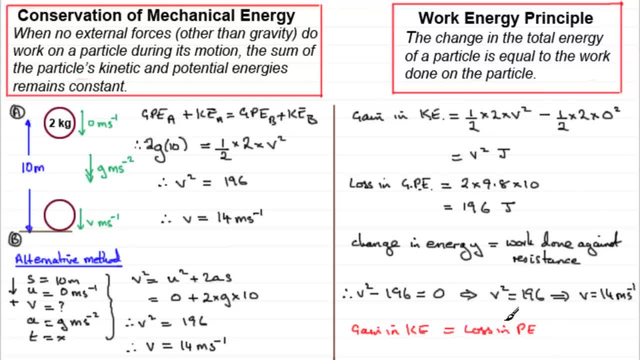 the gain in kinetic energy, v squared equals the loss in potential energy 196.. There you go that line there. So, as I say, you might see this written out by a computer, So you may have to write a little bit of this down. So it's very, very simple. 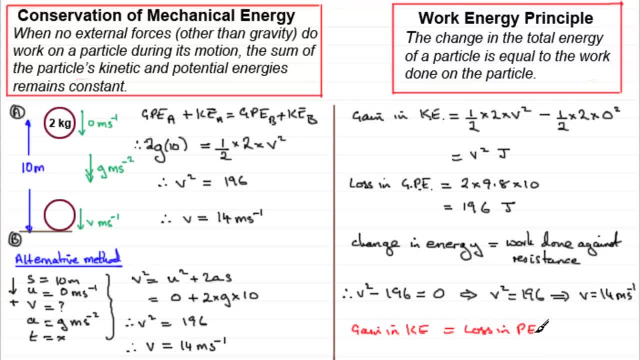 But if you've got a lot of work and you're in a class that's very complicated, a lot of studies of this kind, you might need to remember that the line is the same in some cases. So we have snap graph on the top of the graph, So we're going to go ahead and slide. 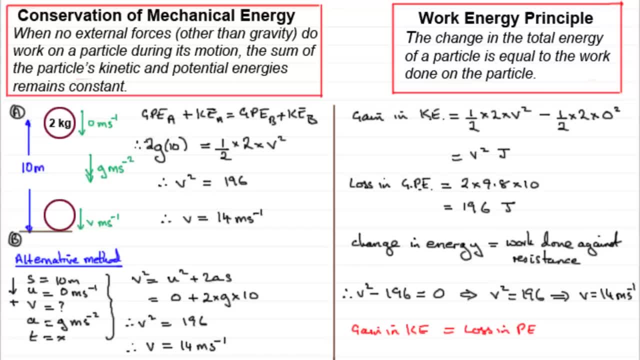 this over here, And now I'm going to do a little bit of this. So it's going to be less than one half of the scale. So that's what I'm going to do, And here's the difference. What's this going to turn out to be? This is going to turn out to be 0.3.. This is going. 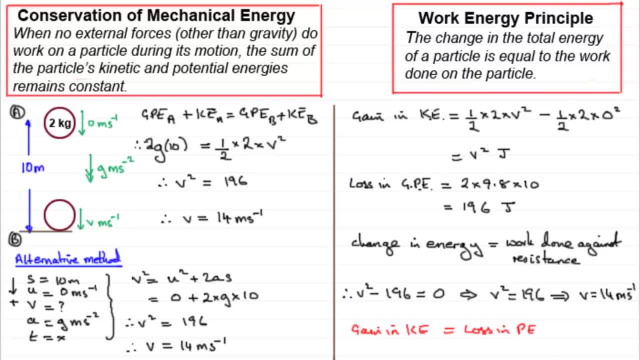 to be 0.3 on the top and this is going to be 0.2 on the bottom And there's no difference. we'll look at other motion that is not necessarily in the vertical plane or in an inclined plane, say a skier going up and down a hill. 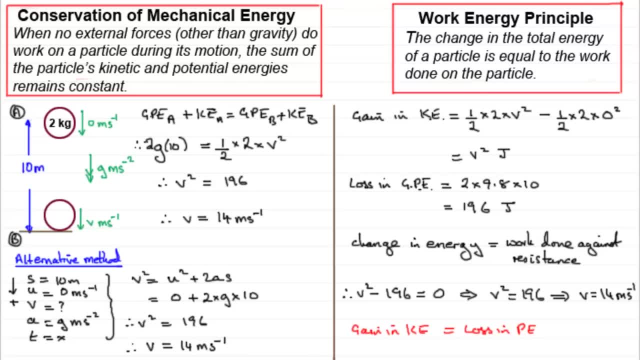 okay, well, that brings us to the end of this particular tutorial, then.